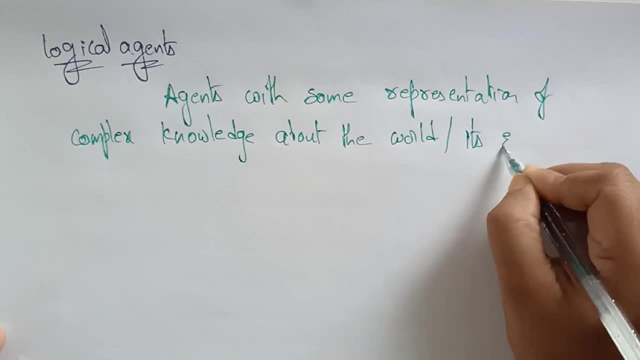 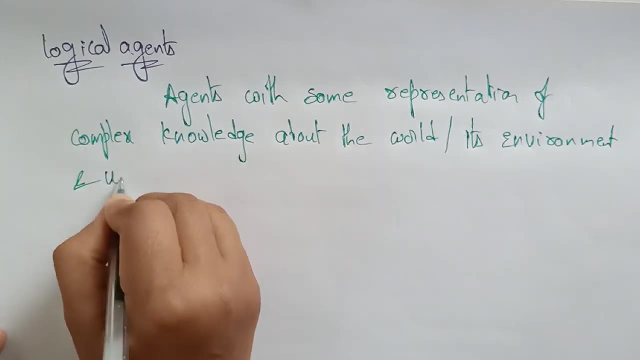 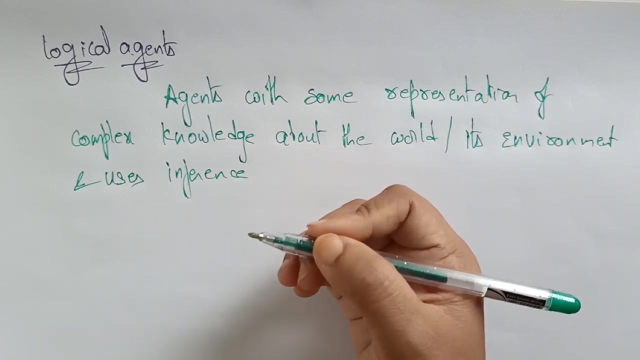 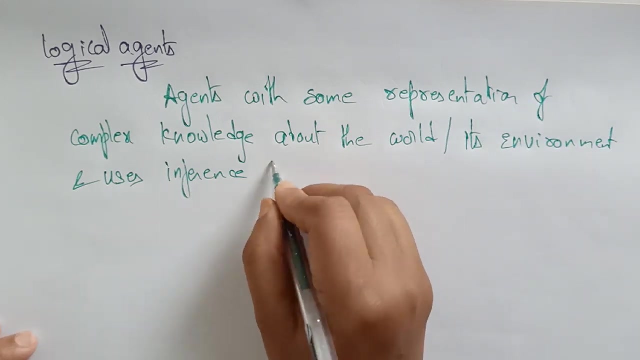 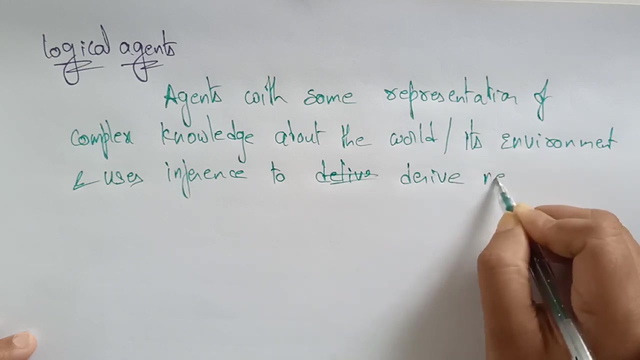 it as about its environment. Its environment and uses inference to deliver and uses inference. Inference is nothing but it is by taking a new inputs with the help of the old knowledge, just taking the new inputs and generating a new concept. So it's an environment and uses the inference to deliver or to derive new information. 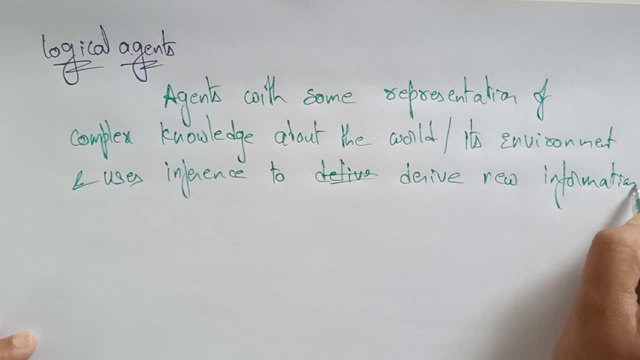 new information, from the knowledge combined with its inputs, From the knowledge from the knowledge combined with new inputs. So the logical reasoning and the information that are present in that can be used for implementing the artificial intelligence. So this is about the logical agents: A logical agents. it's simply. 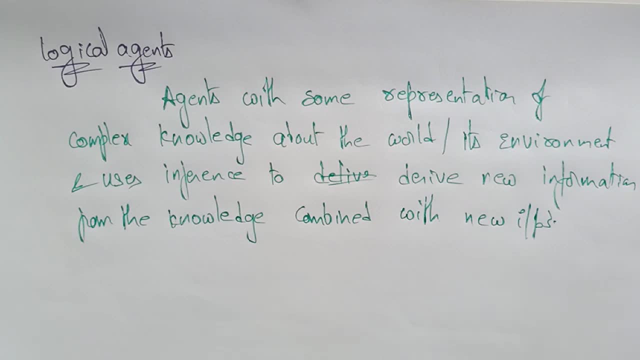 it's you call it as an agent with representation, with some representation, of a complex knowledge about the world or its environment, and uses the inference to derive new information from the knowledge combined with the new inputs. So the key issues here in the logical agents is the 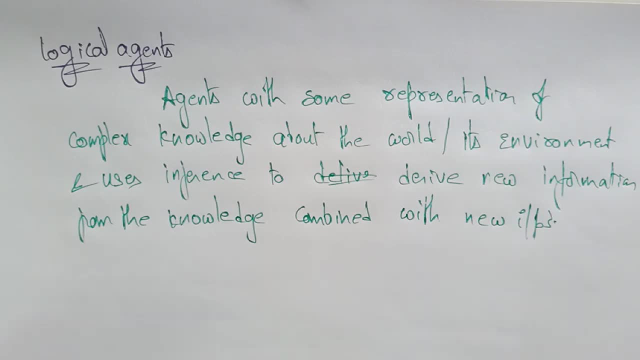 representation of the knowledge and a reasoning. Okay, so it's completely. it's about the logical agents. The logical agents, it's completely based on the knowledge base. So we are talking about the complex knowledge Agents, with some representation of complex knowledge. That means we. it's complete. 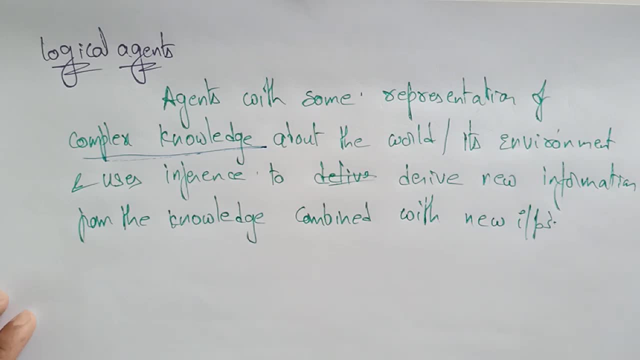 the logical agents is completely based on knowledge base. So what is a knowledge base actually? So before going to enter into the concept, you have to know these terms. Okay, if you know the terms, then you can understand the concept. A logical agents with some representation of. 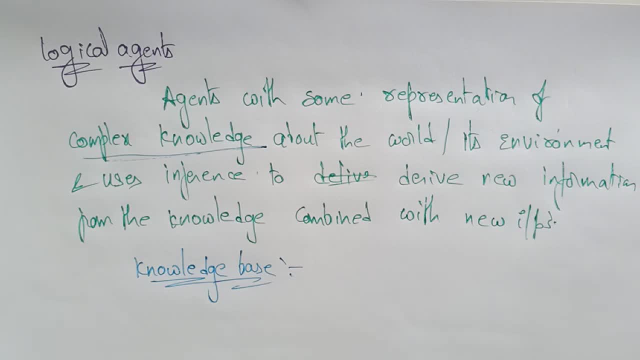 complex knowledge. so we are talking about the knowledge. actually, what is this knowledge base? uh, what the knowledge base? it's just set of sentences in the formal language representation. it's just a fact about the world. it's just a fact about the world knowledge base. it's just. 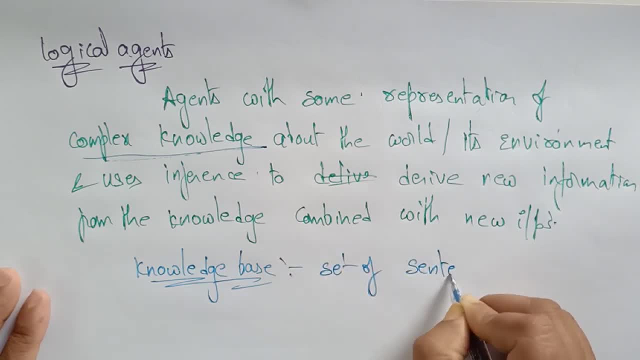 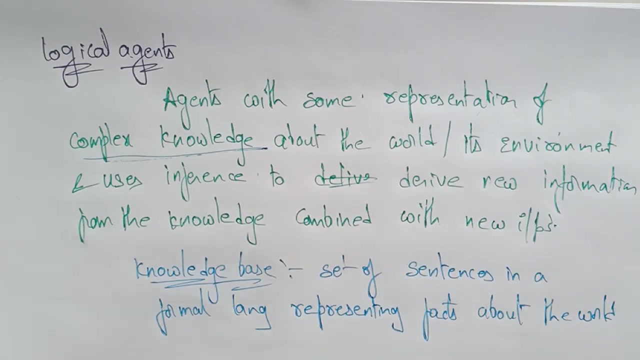 a set of sentences in a formal language. we are representing in a formal language, representing facts about the world. that language is representing facts about the world, so we call it as a knowledge representation. okay, so this is just a small concept about what is the logical agents, and this logical agents are the information that 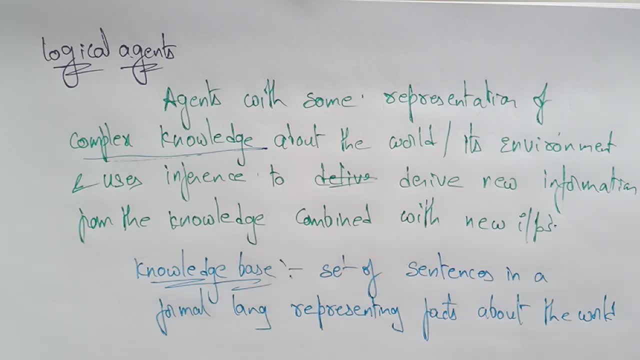 agents is representing of the knowledge. So what is this knowledge? The knowledge completely depends upon the knowledge base. A knowledge base is a set of sentence in the formal language representing the facts about the world. Okay, So let's see what is: knowledge based agents. Okay, So knowledge. 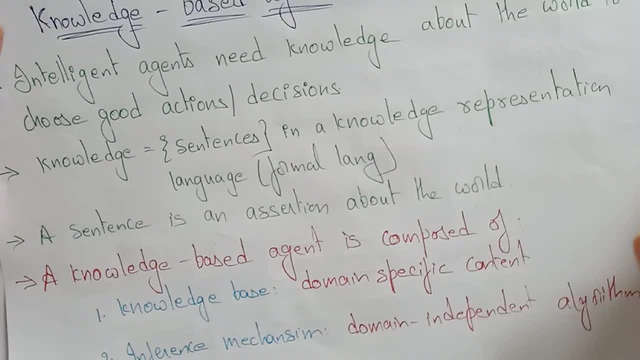 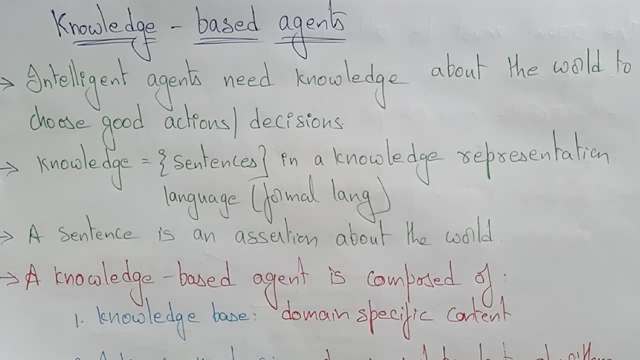 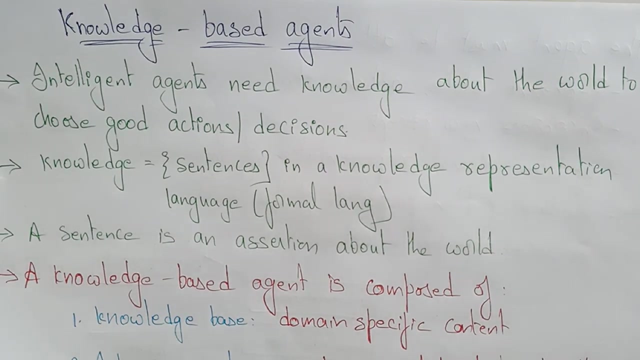 based agents. Let me explain. So I explain: what is a logical agent? So the logical agents is completely represent in the form of a knowledge. So the knowledge should be there to represent everything logically. So we have to know about the knowledge based agents. So what are the? 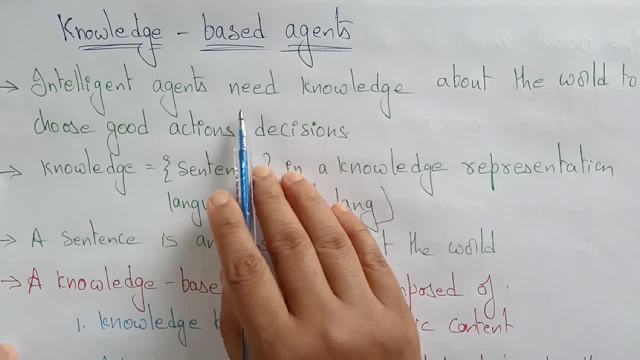 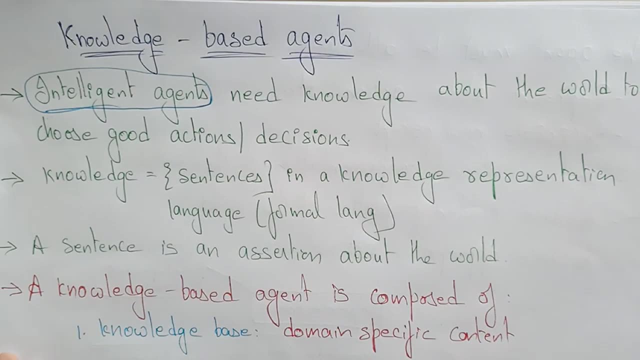 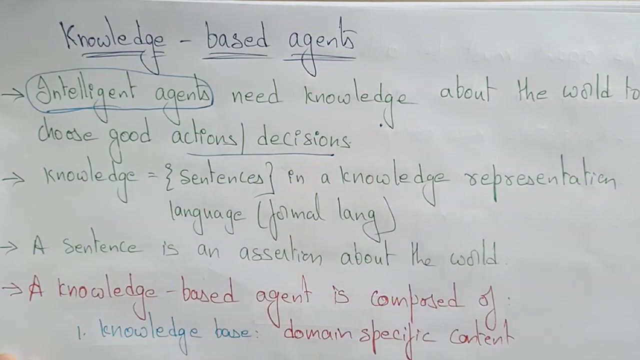 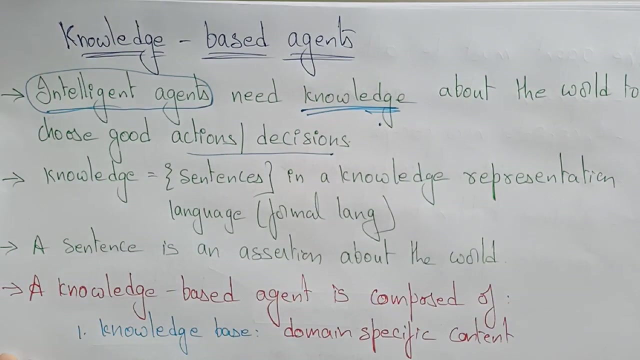 knowledge based agents. Intelligent agent needs knowledge. Obviously the intelligent agent, whatever the intelligent agent, is there. So that agent needs knowledge On what About the world to choose good actions or decisions. If that agent wants to choose good actions or a decision, it needs knowledge. So a knowledge is simply, it's a sentence, It's. 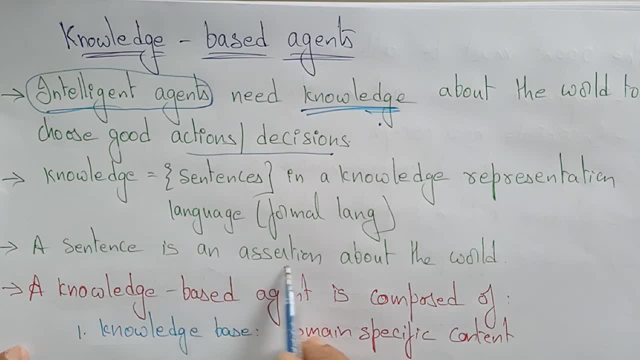 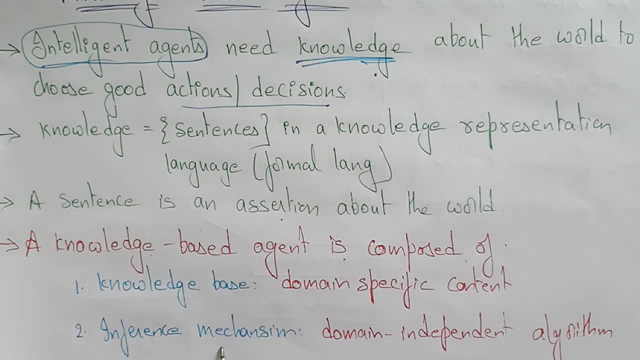 just representing in the formal language. So a sentence is an assertion about the world. So the complete, a knowledge based agent is composed of two parts: One is the knowledge base and another is the inference mechanism. So I already said, inference is nothing but deriving. 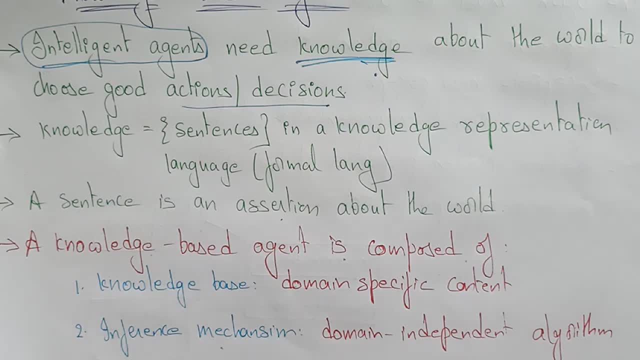 a new sentence from the old. So with the help of the old sentence you are deriving the new sentence. This knowledge base agent is composed of the knowledge base and the deriving of a new sentence, The old knowledge and the new knowledge. So knowledge base is the domain specific content. 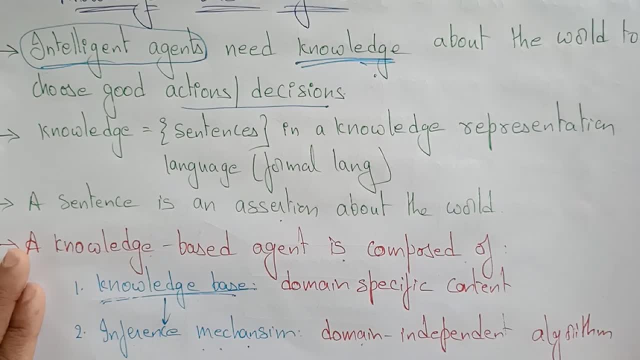 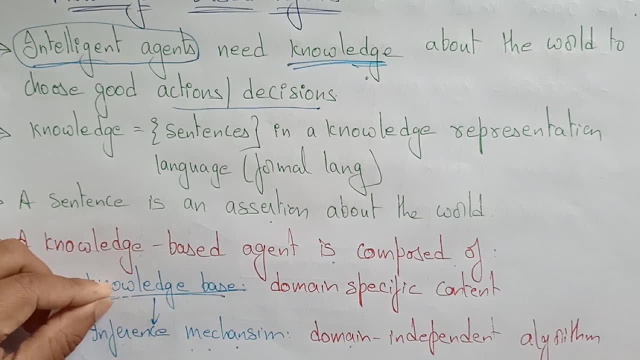 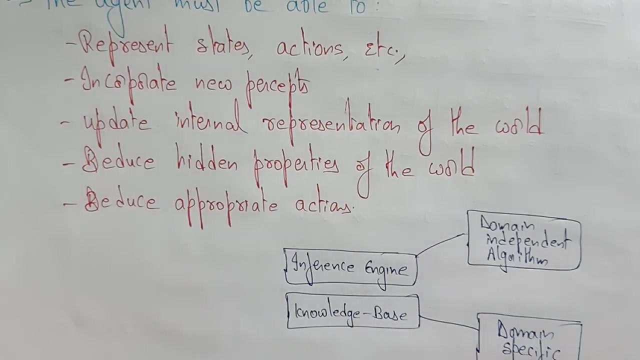 whereas inference mechanism is the domain independent algorithm. So remember this point: A knowledge base agent is composed of knowledge base and the inference mechanism. This is the domain specific content and this is the domain independent algorithm. Okay, So now let's see that agent. that knowledge base agent must be. 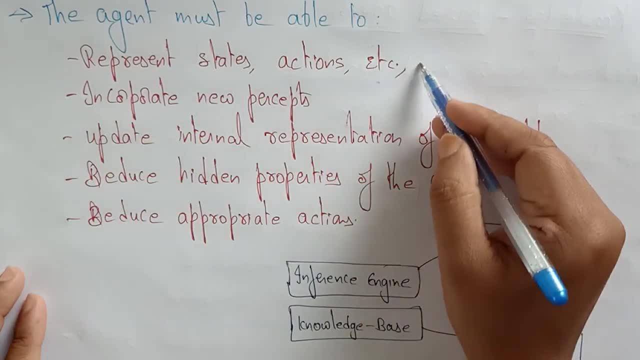 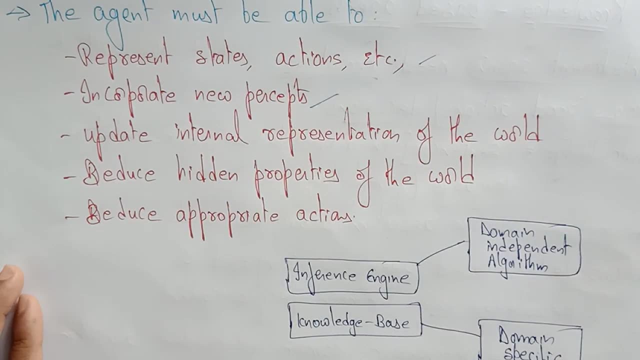 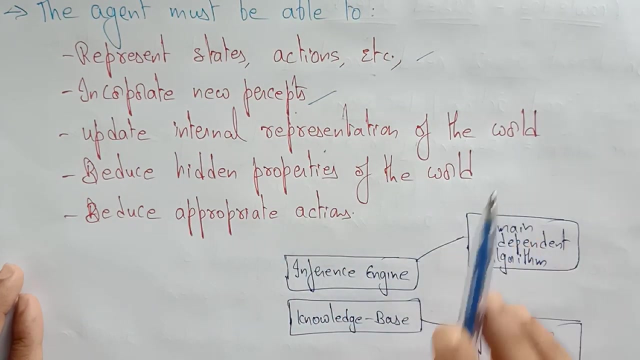 able to. it's nothing, but it must be able to represent the state, actions, etc. And it incorporates a new percepts. Okay, So that is the inference. It's just deriving a new sentence from the old. It's incorporates a new percepts, updates the internal representation of the world, So that 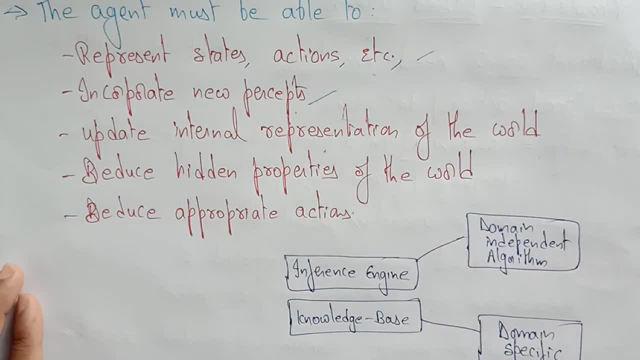 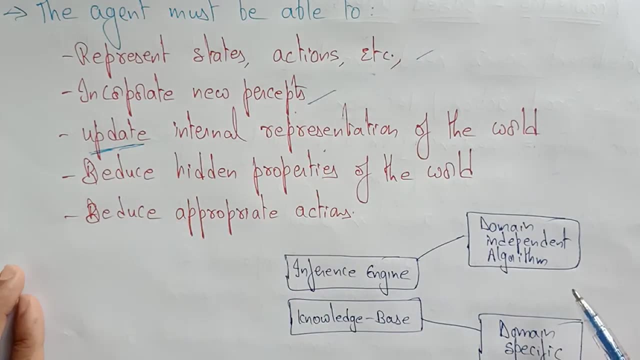 agent which is having the knowledge based, So it is going to update the internal representation of the world. It is going to update the internal representation of the world And it deduces the hidden properties of the world also. Okay, It's world is nothing but the environment. 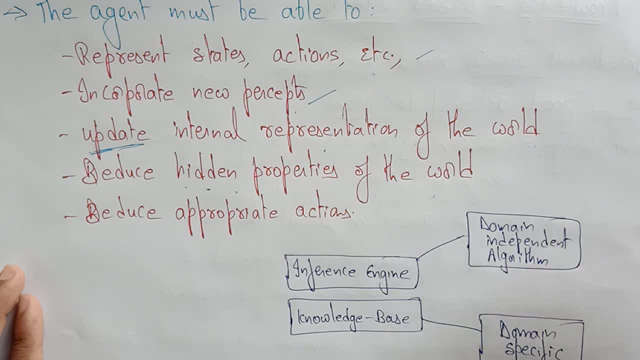 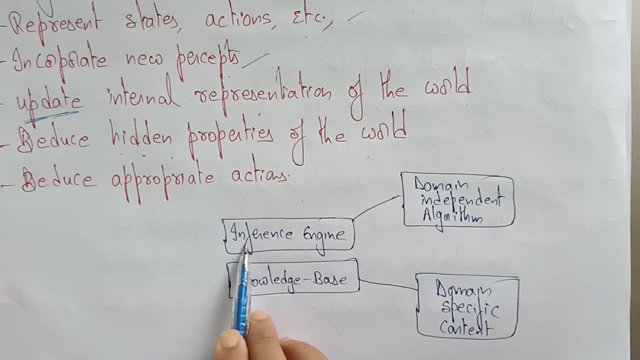 whatever it is dealing, So it deduces the hidden properties of the world and it deduces the appropriate actions also. So you can call. I said the knowledge base is composed of two things: One is the inference engine and another is the knowledge base. So the inference engine is a. 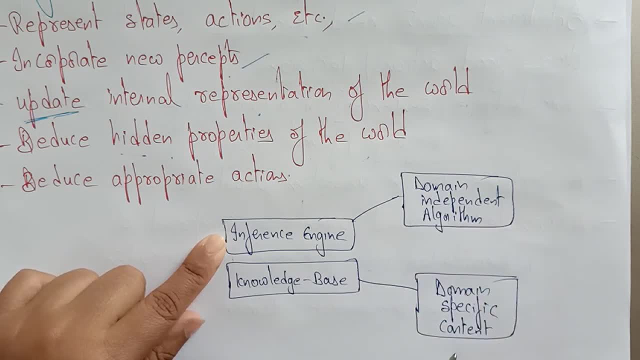 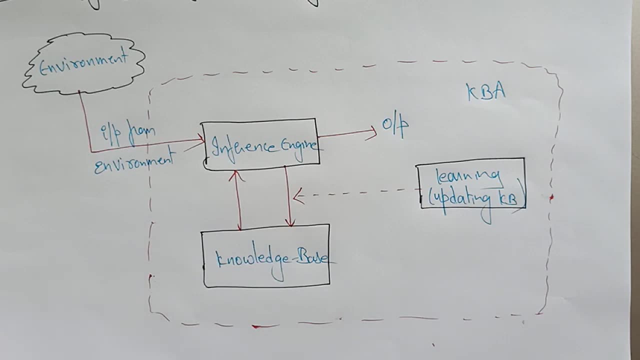 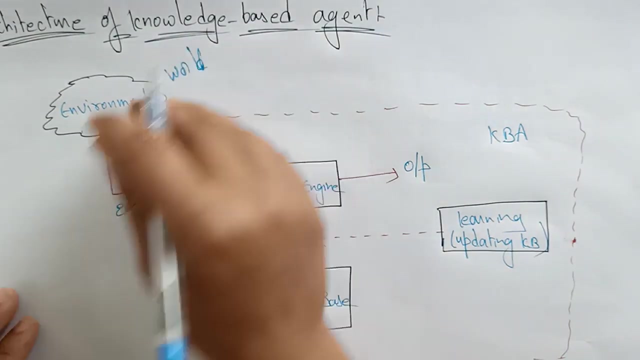 domain independent algorithm, whereas knowledge base is a domain specific content. Let me explain you the architecture of this knowledge based agent. The architecture of knowledge based agent, So I said it's environment, or you can call it as a world. Okay, So this environment, so this completely, is a knowledge based agent. This. 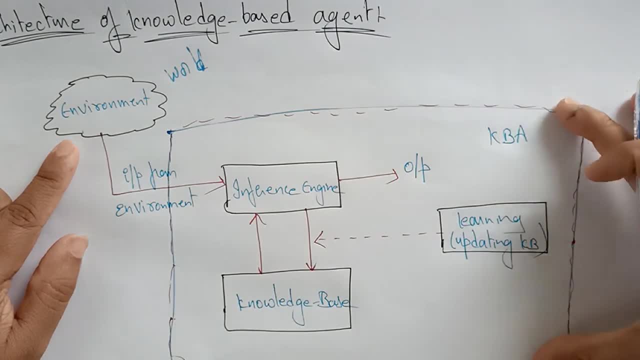 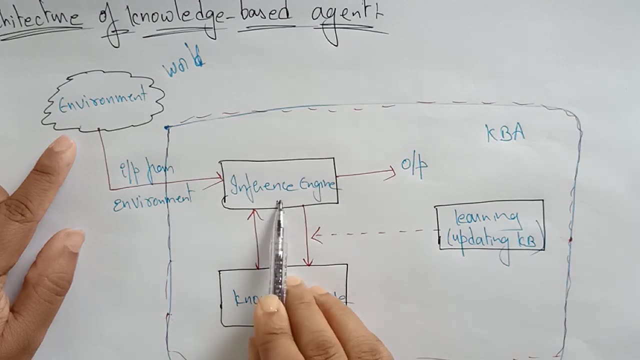 part. you call it as a knowledge based agent. So this is a knowledge based agent. So what does knowledge based agents consist of? It consists of inference engine, which is going to derive a new sentence from the old, So it takes the knowledge base with the help of the knowledge base, whatever. 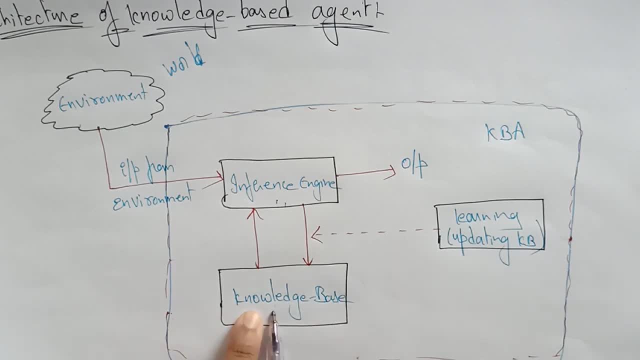 the logics it is having. it's a knowledge base. it means nothing but the logic it is having. with the help of that knowledge logics, it taking the input from the environment. with the help of this knowledge base, it is delivering an output which is a new sentence from the old. okay, so here. 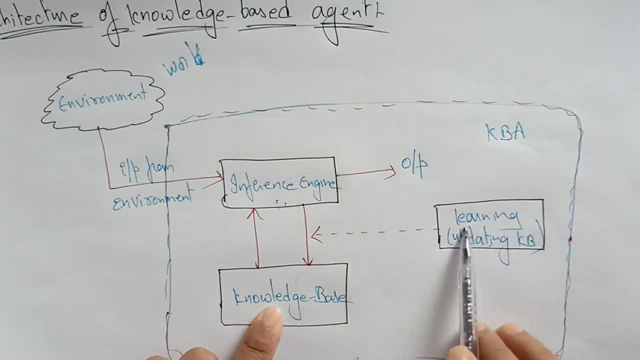 an updating will be there. the updating knowledge base will be there. that you call it as a learning. okay, updating knowledge base. whenever there is a requirement to add some software or any updations you want to make to that artificial intelligence, you can update with the help of.